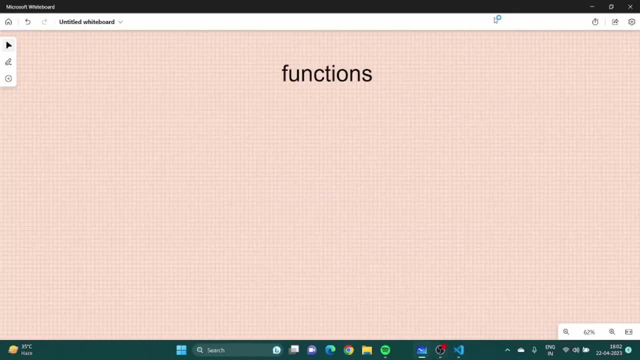 Hello everyone and welcome back to another video of our web development series, and in this video we are going to look at a very important aspect of every programming language that tells functions, So let's try and learn it by an example. Suppose this is your home. 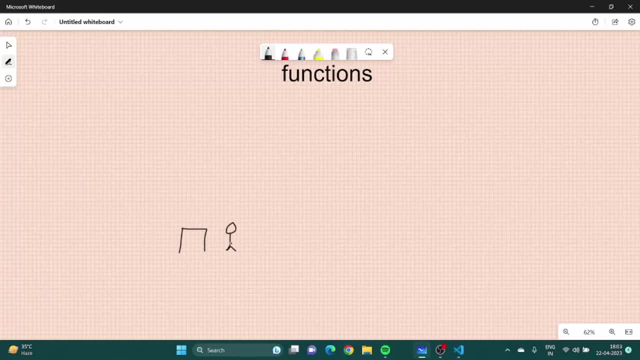 and suppose you have a robot. My drawing is not that good, so don't judge me on that. You have a robot and here there is, let's say, shop. Now what you have to do is you have to program this robot in such a way that it goes to this shop and brings the milk Suppose. 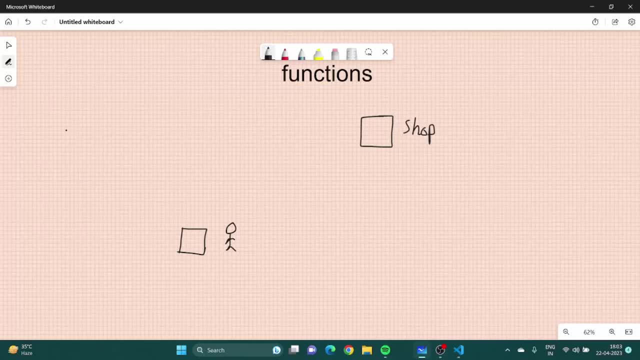 you give it some commands. Let's say exit home- Okay, I am not writing the commands, just giving short forms maybe: Okay, great, Exit home. Then what Move right, Then what Move up By, And then what Move down, Move left, Okay, 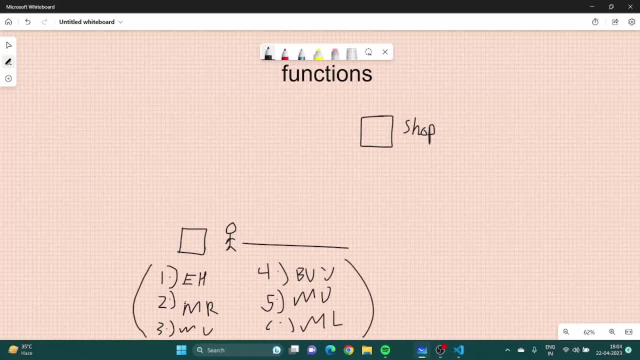 Suppose these are all the commands. Now what would happen? The robot would go to the shop, It would buy something, and then it will come back again to your home and will get the milk. Now suppose you have to do this, like you want the milk everyday, So you have to write this piece of code again and again. 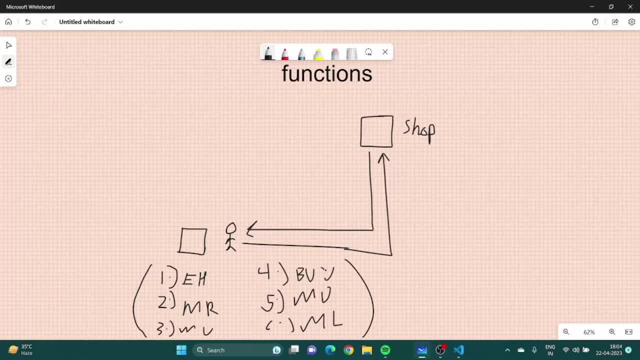 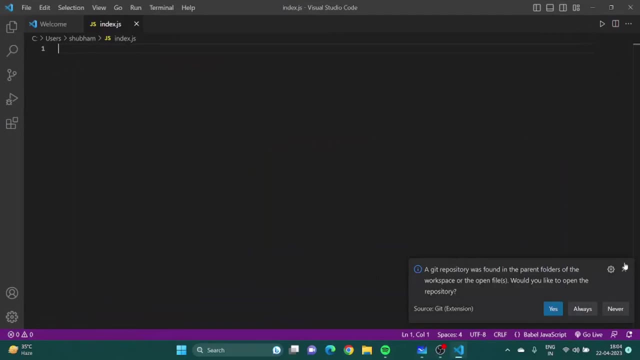 So it is a bit tiring, Right? So for this thing there is something called functions, which we have. Okay. so what does function exactly do? is inside the function. what we do is we write a bunch of reusable codes. Okay, Let's say, functions are a block where we write reusable codes. 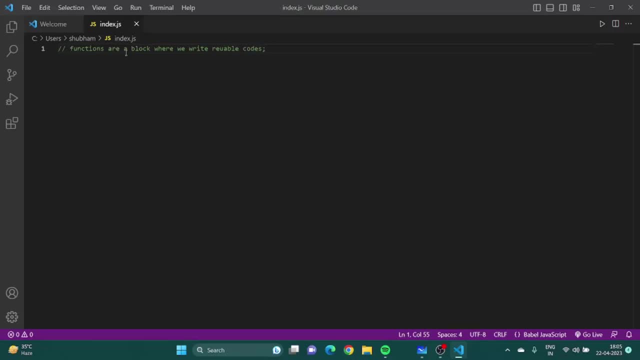 Okay, Okay. So another major thing is you might be wondering: how do we call the function? Simple, We call the function by, let's say, function, and then we write name, or we give it a name to the function. Okay, Like, suppose, what I used to write, I used to write var a and give it something. 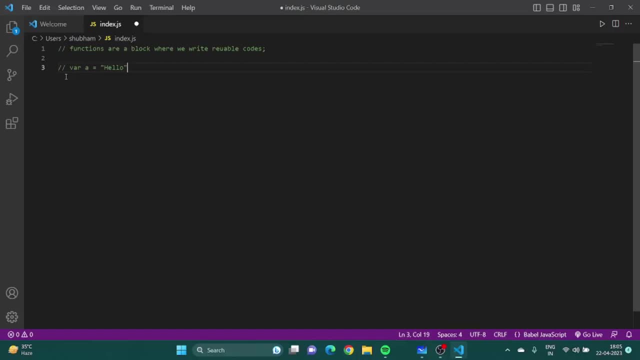 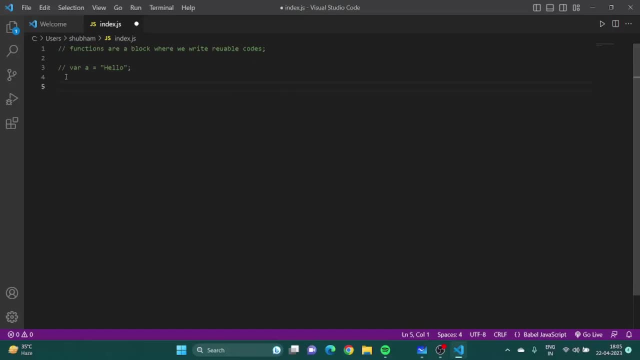 Okay, Okay, Okay, Okay, Okay. Now I need to actually write a function. So I have already a function called employees and I give it a name And I'll tell you why that process was done. Okay, So a function was done, Okay. 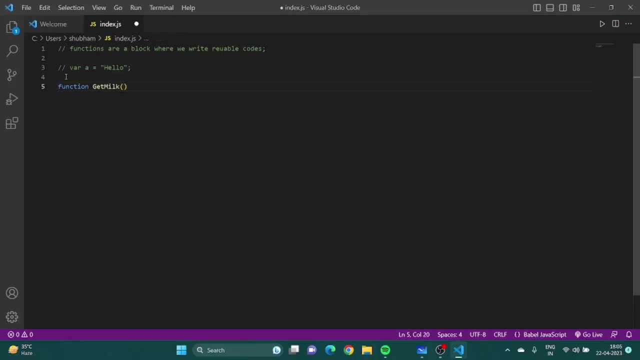 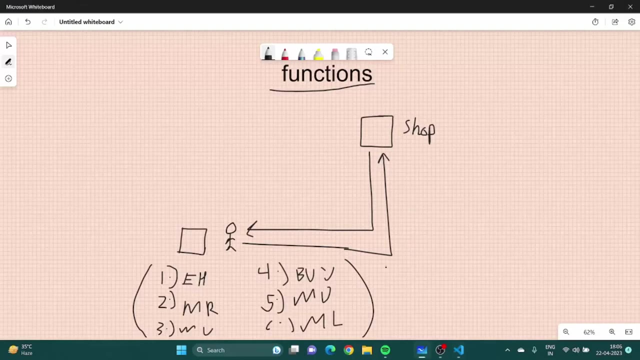 So the function that we are writing was defined. You know what we were doing is. you were put the value Okay And you give it a function Okay. Okay, This function gives us this output. Let's say, if this is the function, mining environment. So this is the way you give the data. All right, See that in this. all this is how I called that Herman Haas block. we give it a call because it is the same way. instead of our, we have to define its function through write function. 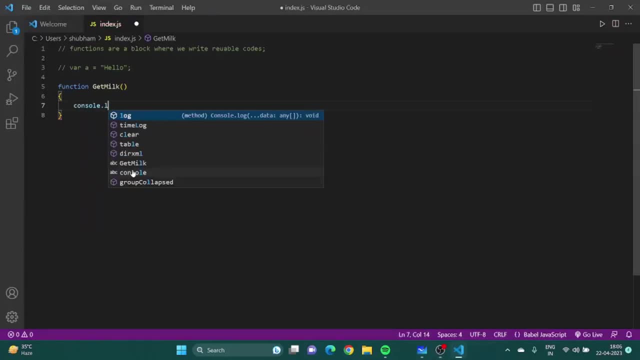 We get a name. let's say: here get milk, we give it a round brackets. I tell you why I write consolelog. what we had in here it was exit home. okay, let's say exit home, and then the consolelog I'll say move left. then I'll say move up. 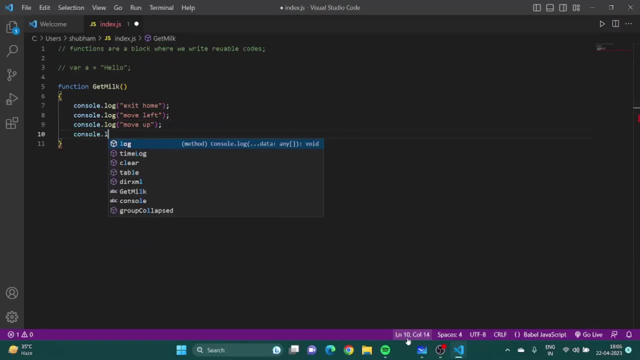 then I'll say get milk. then I'll: okay, let's just keep it this. you can complete it all when you have the time. but okay, now what I'll do. how to call this function. similarly, I'll just say get milk, and this is how I call the function. 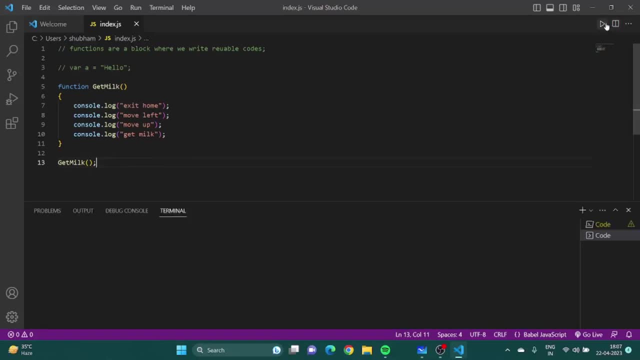 okay, now, if I click on this run button, let's see what the terminal would show: exit home, move left, move up, get milk. if I remove this and if I save it, nothing happened because I'll define the function, but I haven't put anything inside. I mean, I haven't called the function. 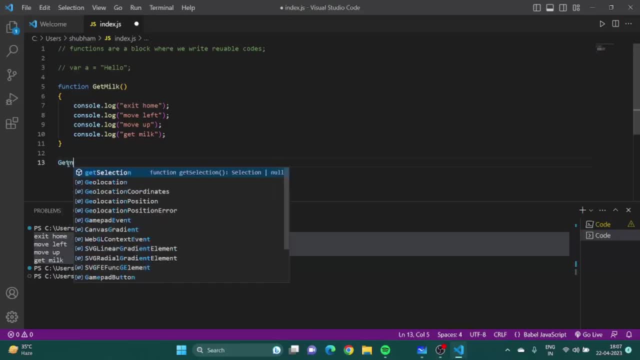 so how I'll call the function? by just writing the function name with the round brackets, and I got it again. okay, great. now you might be wondering: okay, everything is fine, but why do I have these round brackets? so again, I'll give you another example because you understand a bit better with: 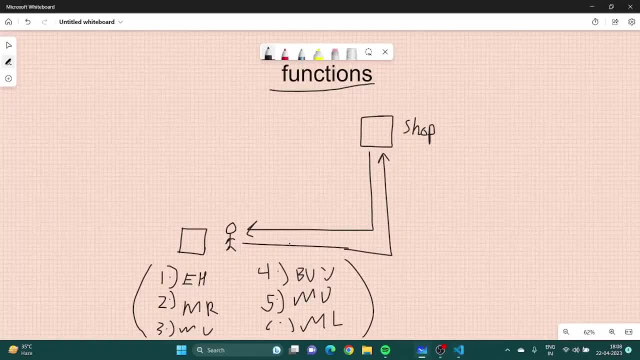 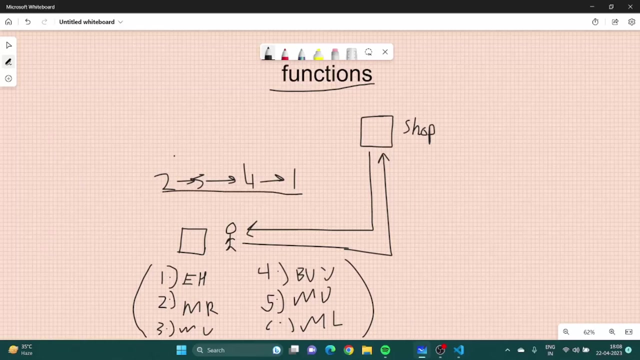 the example parts. now you have this robot and you want to buy milk every day. but suppose on one day you have to buy two packets of milk, but another day you want to buy three packets of milk, but another day you want to buy four packet, or one day you want to buy one packet, okay, so how will you tell the robot this? I mean, 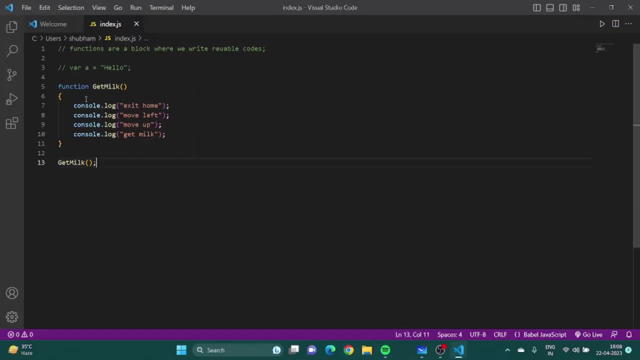 suppose this is the basic function I wrote. but here, where I can tell it right, I mean you have to go inside the function and change it every time. use, let's say, get milk, and we'll define the packets number in packets, let's say: but whenever you call this thing, 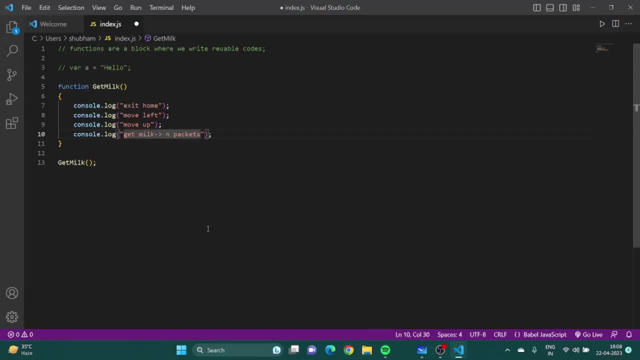 you will always get this amount of packets right. so how to tackle that? so for that, we have these round brackets. inside these round brackets we give them some arguments. okay, suppose I write a varen here and I give it a number, let's say three. it was supposed to be varen. why is it not working? let's see. 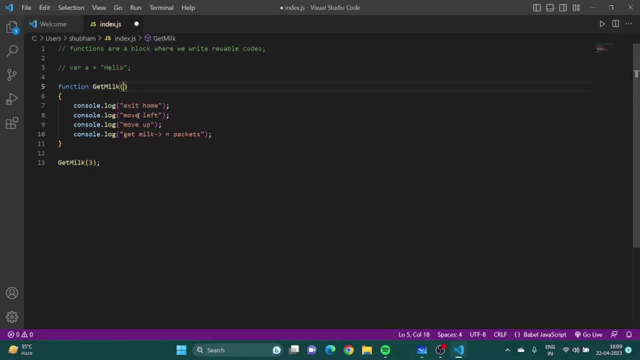 okay, we can give it only n. okay, let's say packets. so what would happen? this three here would go into this packet and then we can use this number anywhere over here. So what I'll do? I'll put this, I'll put this and I'll put a plus sign over here and I'll say packets and I'll put a plus sign over. 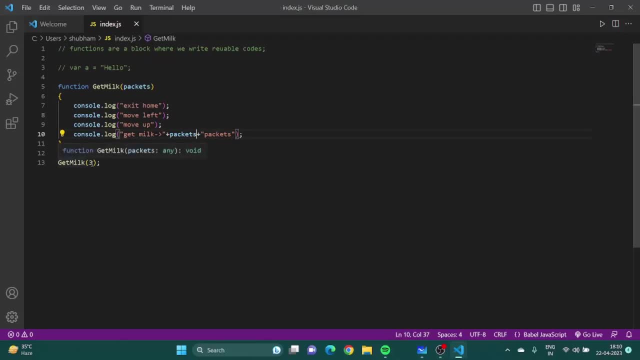 here. Okay. So what would happen? whatever argument I give inside this function- 3,, 4,, 5, whatever number of milks I need, I'll just give it over here- It would go into this packet, and then this packet can be used anywhere in our code. Okay, suppose it's 3 right now. 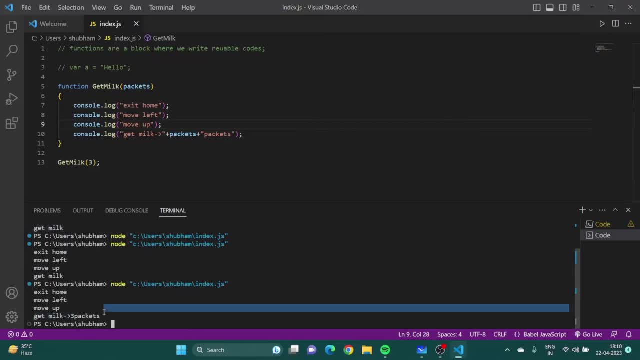 I run it and you can see: okay, get milk, 3 packets Works. Let's just close it and then suppose I write 5, I save it. I have made the run. Okay, 5 packets. Let's put a space there over as well to get it better. Okay, 6 packets. Okay, You see. 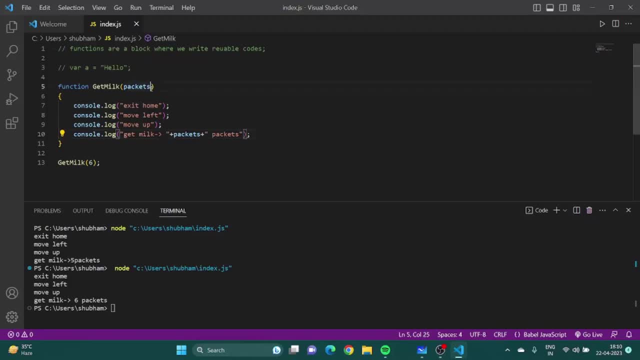 how we pass the arguments and this thing. I can have any number of arguments as I want. I can write 4,, 5 and suppose I give them n, x. Okay, I'll just simply consolelog. let's say n plus x. So what would be the output? 9 should. 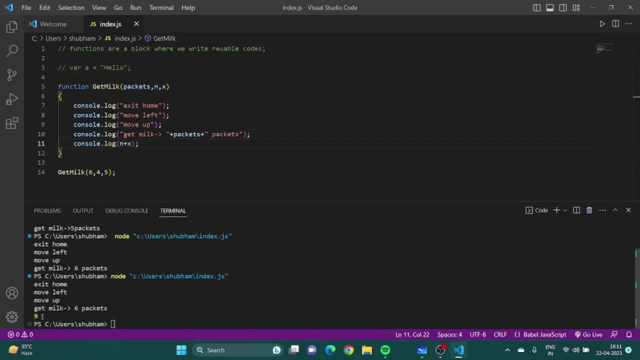 be there. Great Works, Yes, Okay, Nice, nice, nice, nice. So this was all about. you know the functions and I hope you understood the importance of function, because many times in your code you have to like have a bunch of reusable codes. 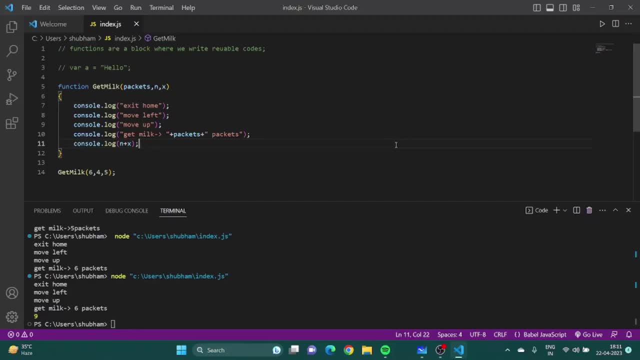 Bunch of reusable lines which you want to, you know, insert in your code somewhere. but obviously you cannot write it again and again because it would be a tiresome process and your code would look very much cumbersome. But here, after this, it looks nice Right. 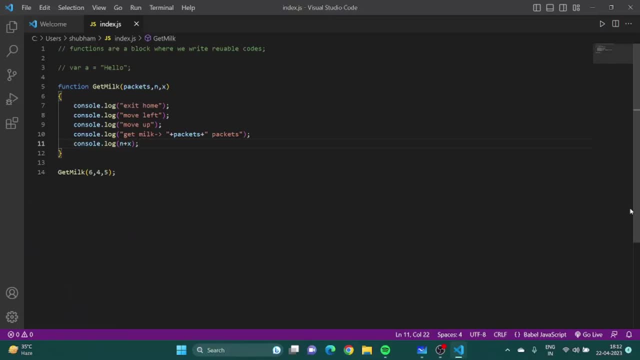 Okay, Great. So I guess that was all for this video and thank you for watching and see you later.